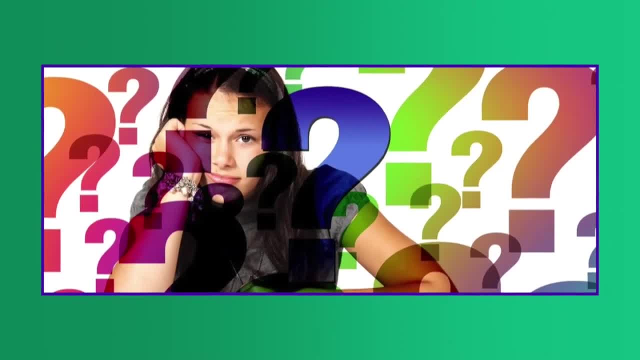 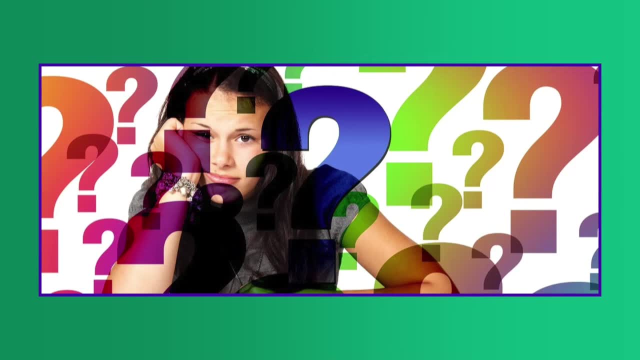 However, language can also be a bit misleading, especially to those looking from outside a culture, like many geographers often do. For example, the default language that many people speak in the area traditionally thought of as Latin America is Spanish, If you were. 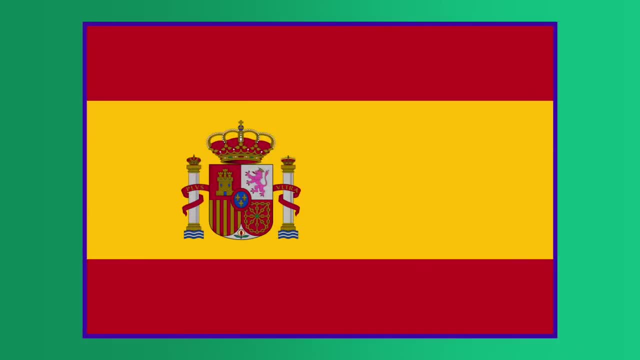 to take that at face value, you might assume that most people came from Spain or have a direct connection to Spanish culture. right Well, as a geographer in training with a little experience already, you hopefully know better by now. Let's explore the varied. 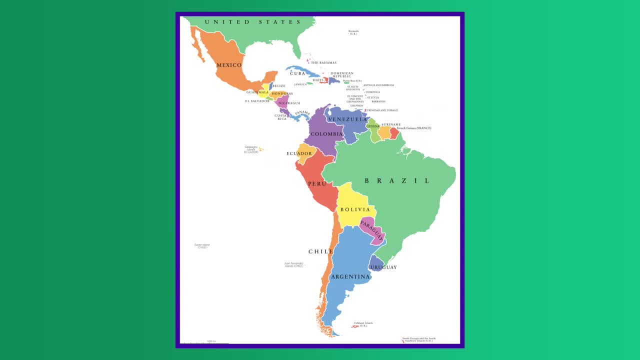 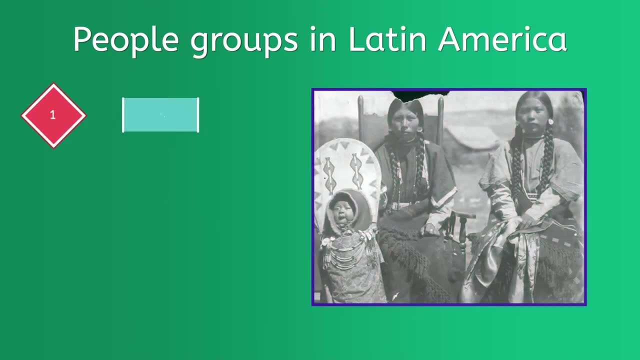 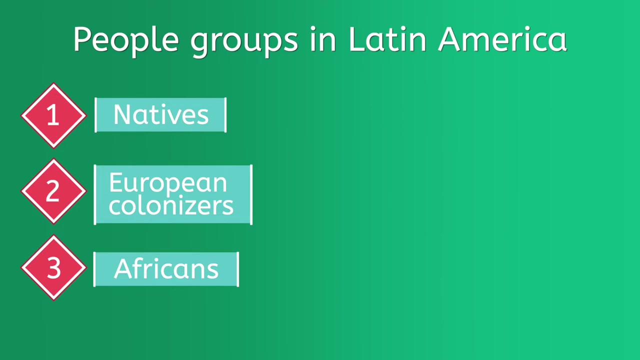 and very different peoples and cultures of Latin America In a very broad sense. we have three major breakdowns of people groups in Latin America. We have the native peoples, the European colonizers and the Africans brought to Latin America against their will as slaves. Now we will add a couple more people groups to this list. 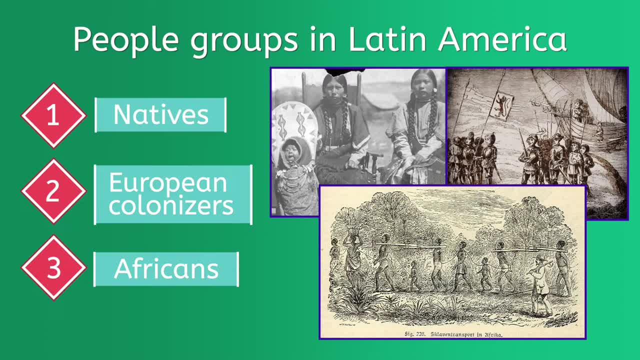 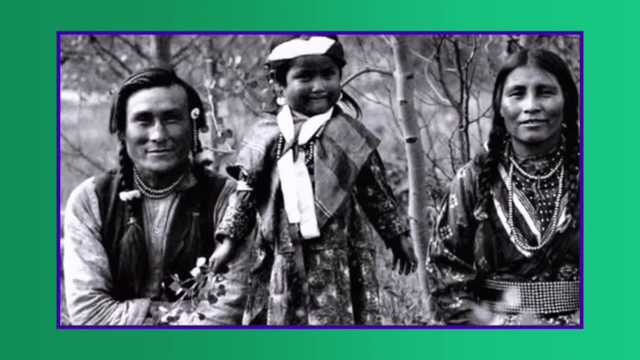 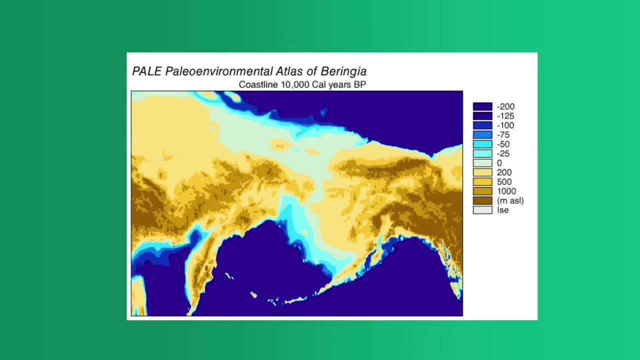 here in a moment, but let's first address where these three people groups came from: Native peoples: It is generally agreed that all native peoples in North, Central and South America are thought to have migrated across Beringia, the land bridge which connected. 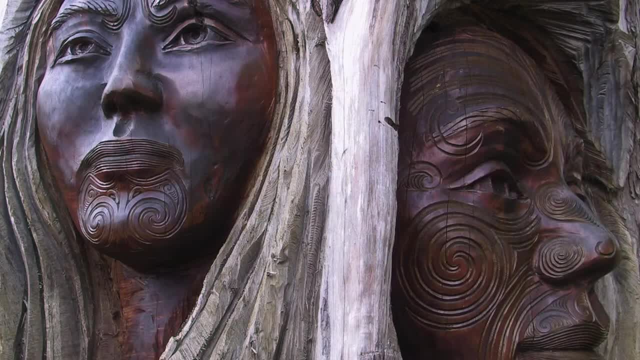 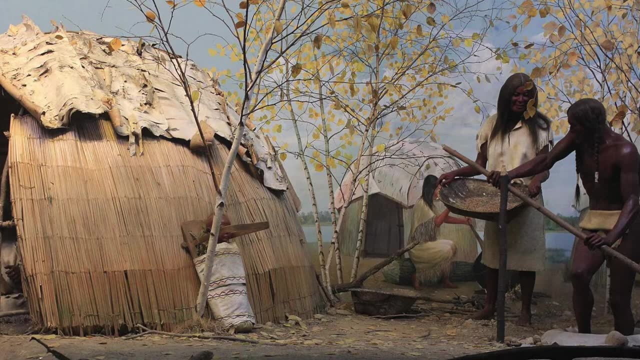 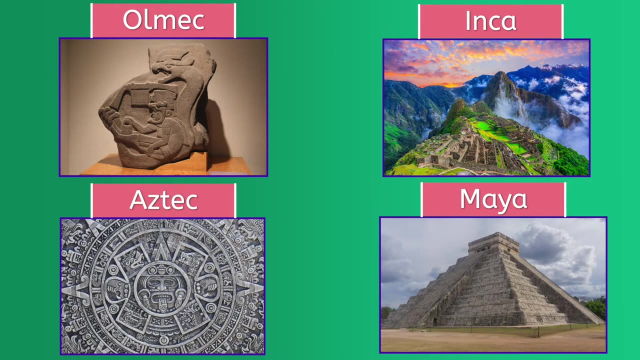 present-day Russia with present-day Alaska. starting as long as 35,000 years ago, These peoples spread across North and South America over time, creating notable cultures such as the Olmec, Inca, Maya and Aztec. Each of these empires developed a unique and unique. 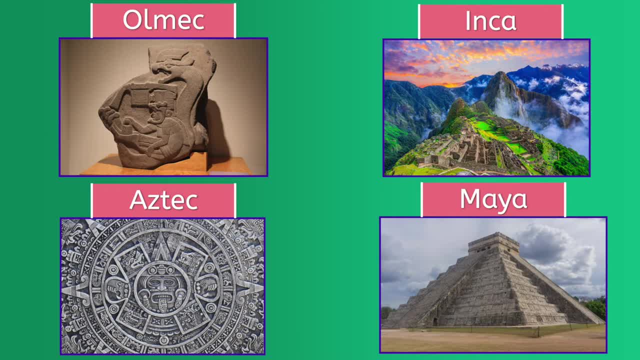 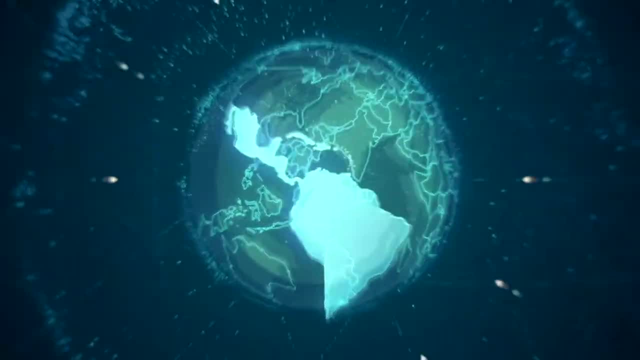 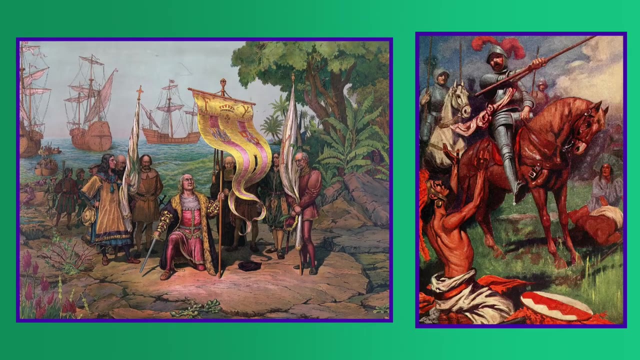 structure, language and cultural complex which, as we'll see in later lessons, still have a major impact on Latin American culture today. Europeans, Beginning with Christopher Columbus in 1492, European conquistadors, colonizers and explorers. 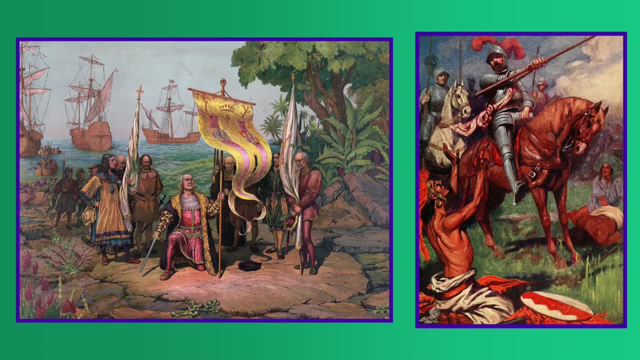 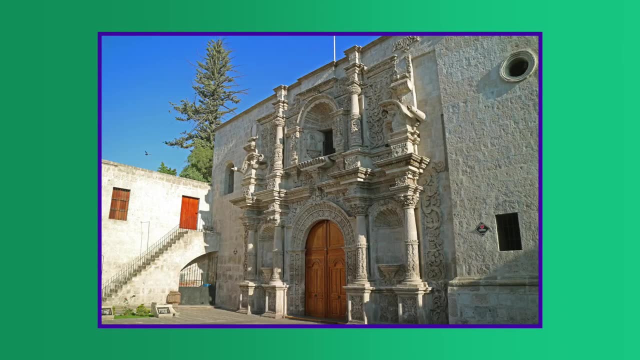 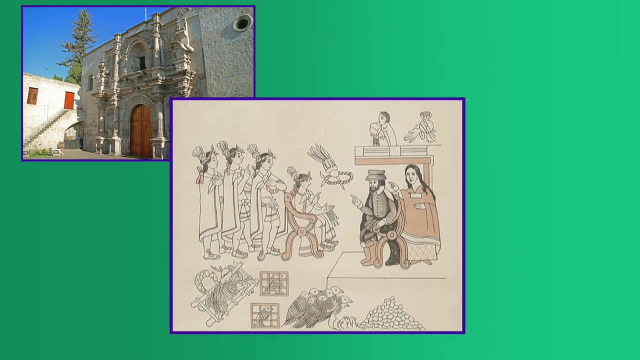 moved into Latin America and by the late 16th century or the 1500s, most of Latin America was under the control of Spain or Portugal. Portuguese established new cities and fortresses and killed or enslaved much of the native population, which did not succumb to diseases brought by their European conquerors. Those 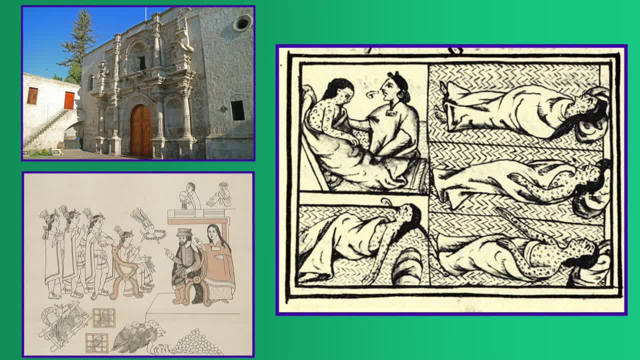 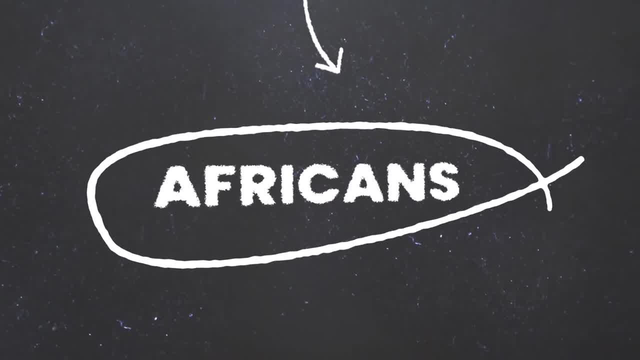 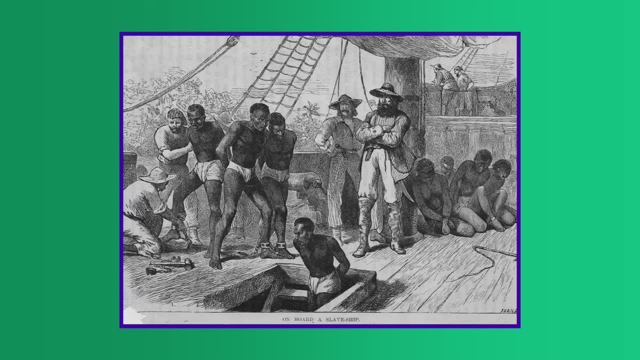 native peoples who were left were not enough to be the slave labor backbone of these conquered territories, and so the Spanish brought in Africans. From roughly 1506 through 1866, an estimated 8 to 12 million Africans were brought across the Atlantic, with an estimated 3.5 million Africans. The Spanish were the first to leave the country and the Spanish were the first to leave the continent. The Spanish were the first to leave the continent, with about 2.5 million Africans left. This massive influx of forced labor also brought east and central African culture with it. 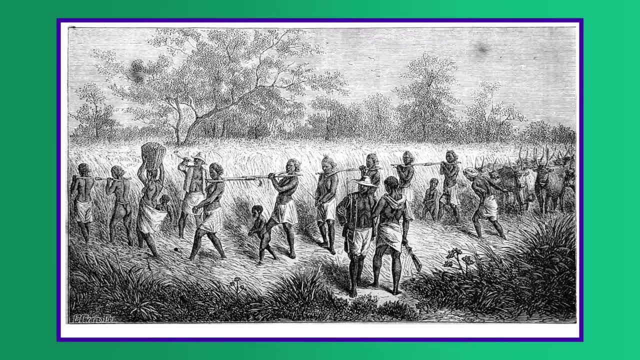 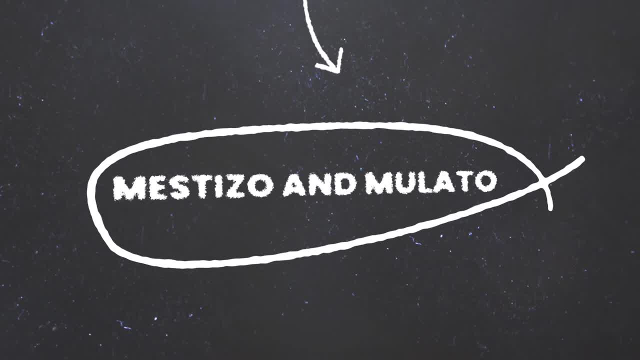 which mixed into many features of Latin American life, an idea we'll explore more fully later on Mestizo and Mulatto. For a hundred years or more after conquest and colonization, Europeans would make racial and ethnic distinctions based upon a pretty simple idea: There's us, the Europeans, and 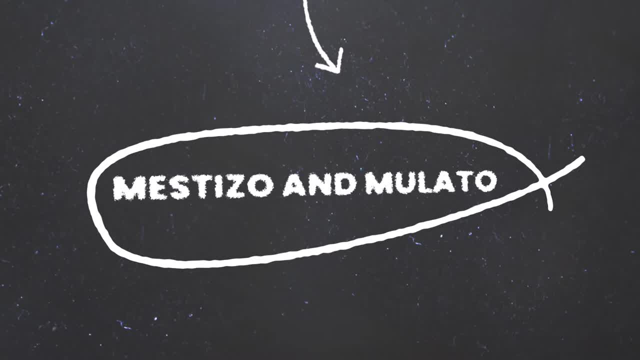 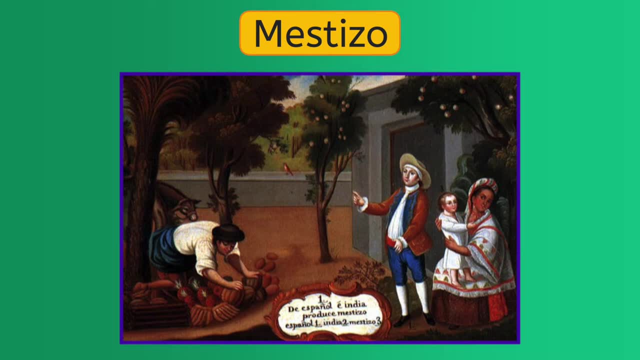 everyone else, everybody else. However, not too long after colonization, the emergence of children born of a European parent and an indigenous parent gave rise to the category of mestizo, This word, which is used widely around the world and for many different groupings and categorizations. 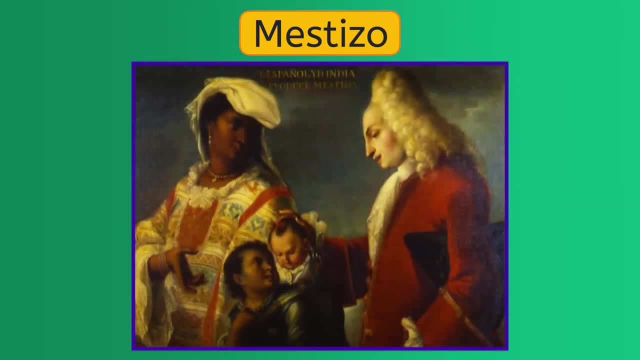 meant in Latin America a person who was of indigenous and European ancestry. In some countries, such as Mexico, this mestizo status created a new culture which eventually rose up and overthrew European control. In other places it has been used in a negative context to. 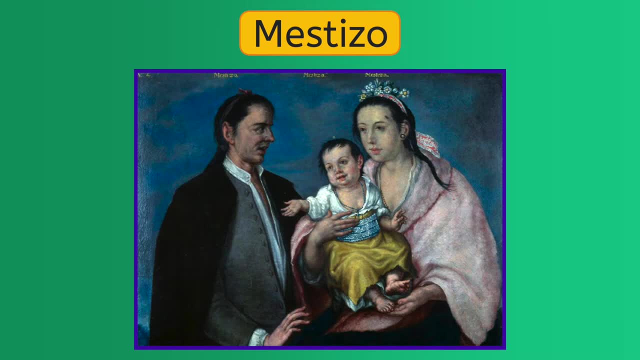 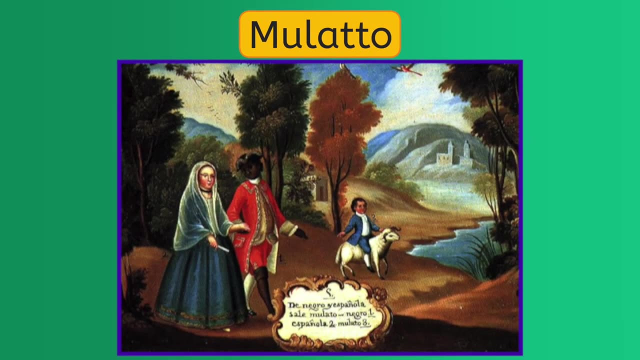 artificially separate people. Nevertheless, an estimated 40% of people in Latin America are of mixed European and indigenous ancestry. The term mulatto, often used for separating out people as often as mestizo, is meant to refer to a person of African and indigenous ancestry. The number of 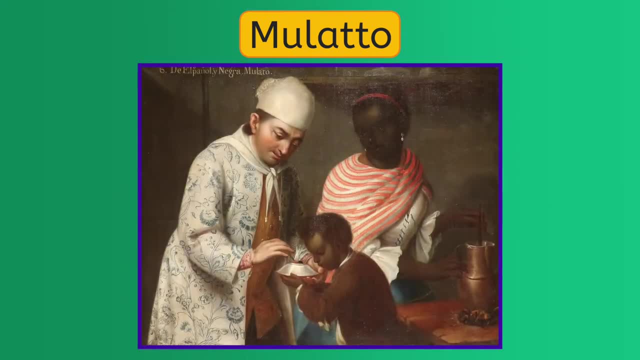 people. identifying with this category varies widely, as it has often been used in a negative connotation. But what does it mean? It means that a person of African and indigenous ancestry was born in Latin America. Recently, more people have proudly identified themselves as coming from. 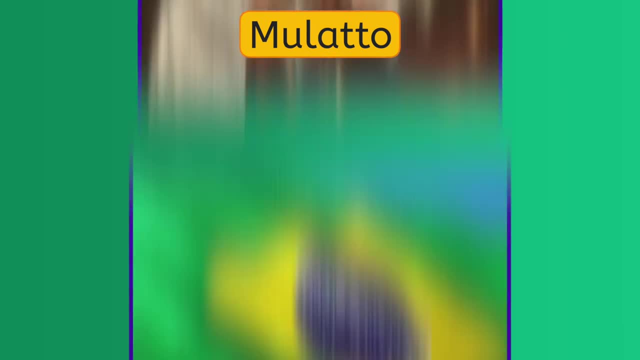 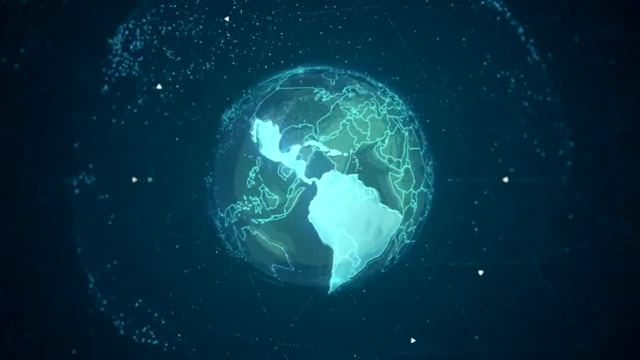 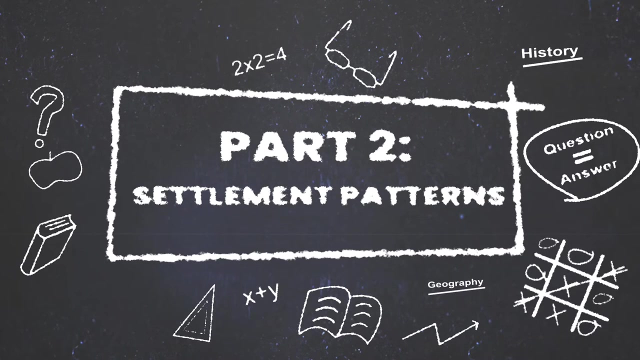 multiple ancestries. Indeed, the vast number of African slaves in Brazil alone have greatly impacted the incredibly unique Brazilian culture seen today. Part 2. Settlement Patterns. So we've talked a little about who lives in Latin America, but now let's answer the question of 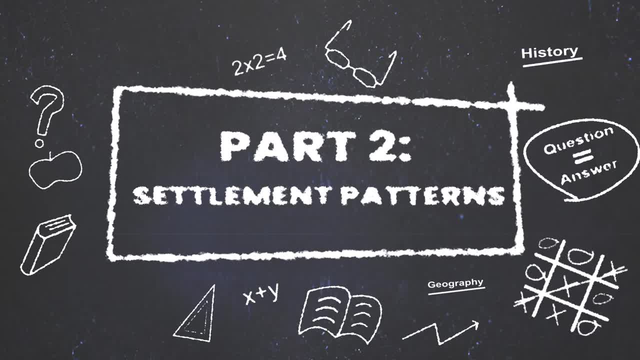 where they live. As with almost all human settlement across the world, most people in Latin America originally settled near the border of the United States and the United States. As with almost all human settlement across the world, most people in Latin America originally settled near the. 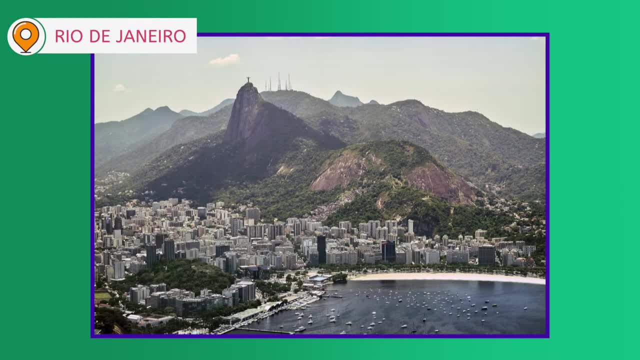 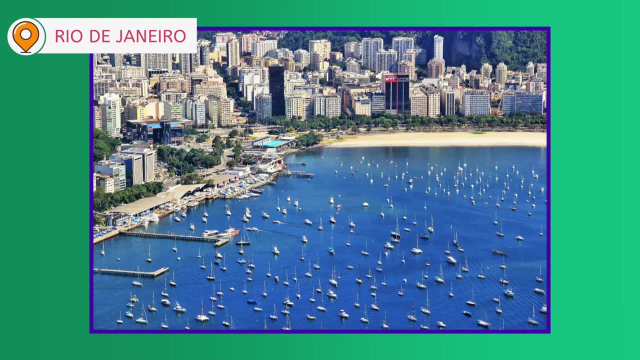 coast or close to rivers and lakes, as these features were then, and remain today, absolutely essential highways of commerce and transportation. It isn't all the same, however. A very unique thing about certain cities in Latin America is their elevation, and there's even a forward capital in. 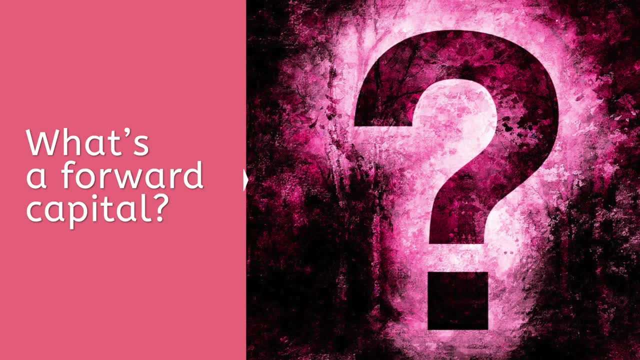 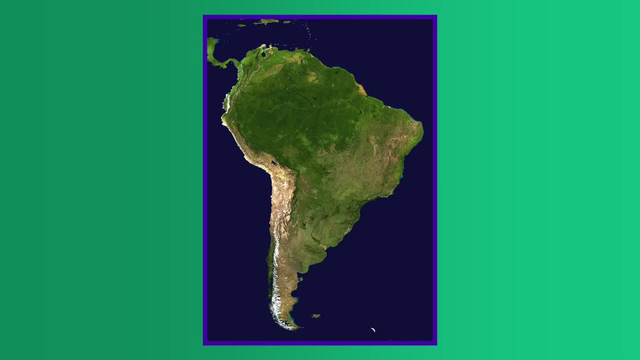 Brazil. What's a forward capital, you might ask? Well, let's find out. First, let's talk about the really highly elevated cities of South America, and there are a few. The highest city in South America is La Oceana, which is the highest city in the world. The highest city in South America is La Oceana, which is the highest city in the world. The highest city in South America is La Oceana, Riconada, Peru. Sitting at an altitude of over 16,000 feet, the city is home to almost 50,000. 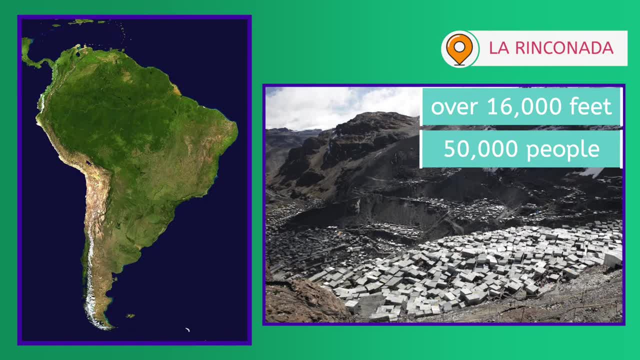 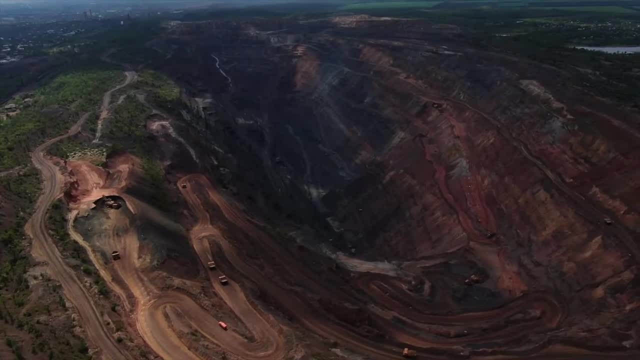 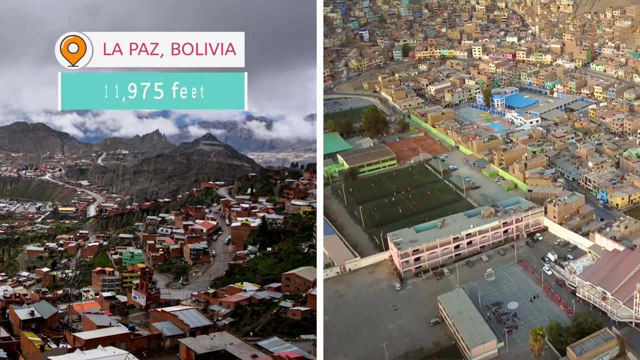 people, most of whom make their living from the nearby gold mines. In fact, many of the highest elevated cities of South America are in the Andes and located near a mine, which is the reason most of them exist. On the other hand, both the cities of La Paz, Bolivia, at 11,975 feet, and Cusco, 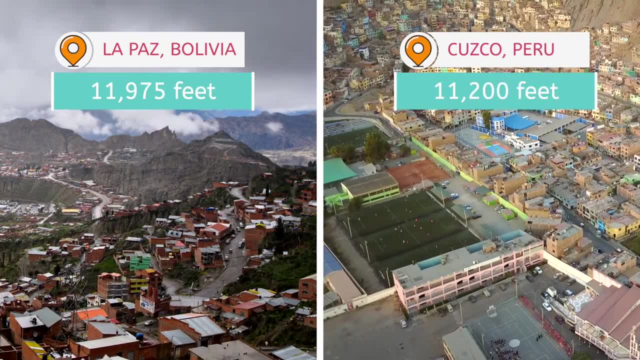 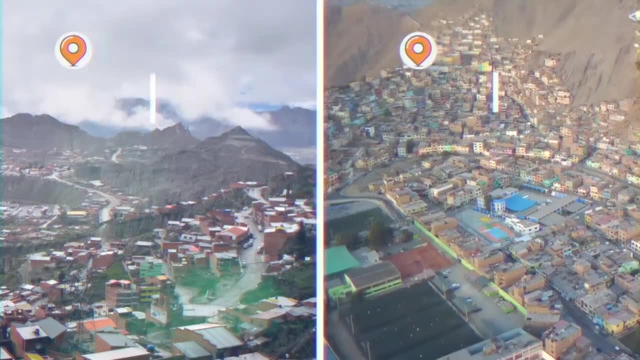 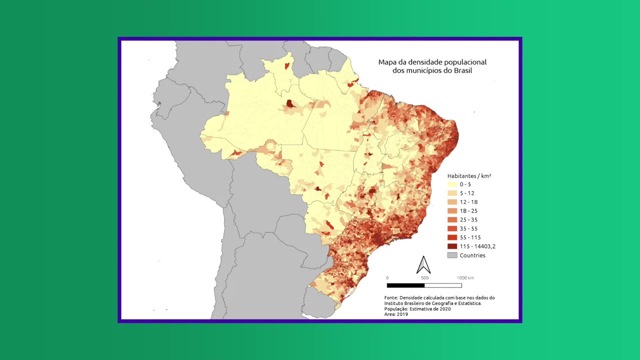 Peru, at 11,200 feet, were previous Inca settlements. The highest elevated cities in South America are, and part of the Inca Empire's vast trade network, Cusco was actually the capital of the empire for a time. Most other cities are built in lowland valleys and near the coast or rivers, as you. 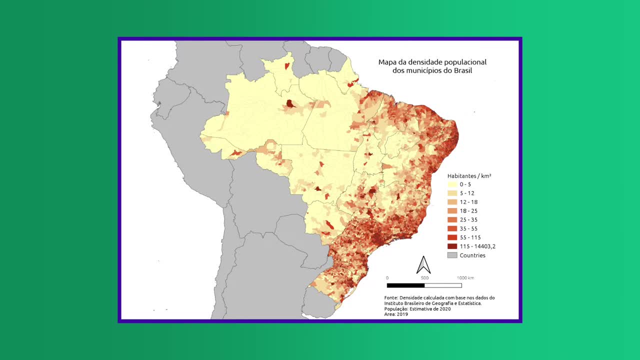 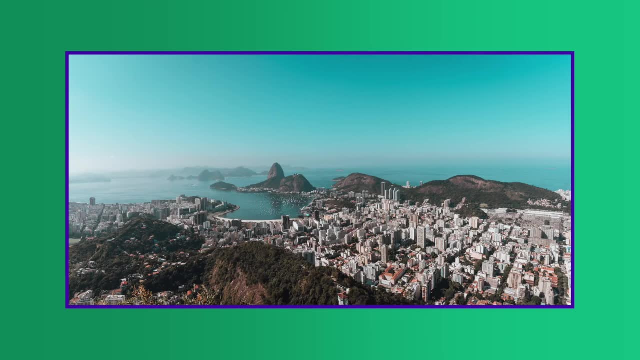 would expect, Many of Brazil's main cities are built along the central coast. These were the locations set up by the Portuguese colonizers for trading the vast amounts of, among other things, sugar cane which was grown in Brazil and, of course, the millions of African. 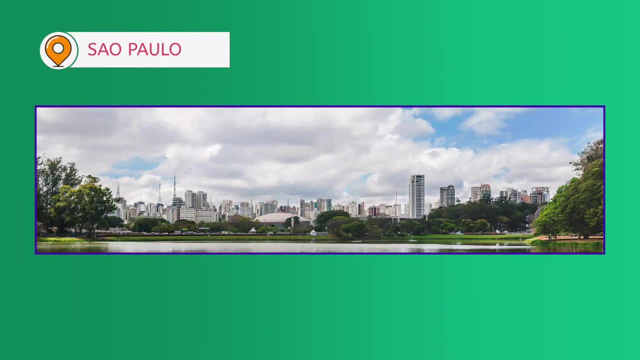 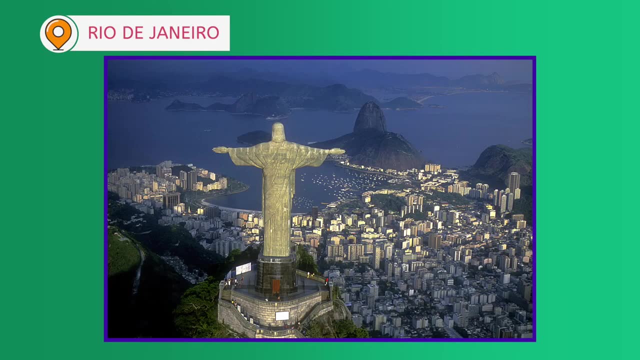 slaves imported to grow it. Sao Paulo is the largest of Brazil's cities by population, and its sister city just up the coast, Rio de Janeiro, are both situated on areas with deepwater ports and are the drainage point for hundreds of rivers flowing into the ocean from the Amazon. 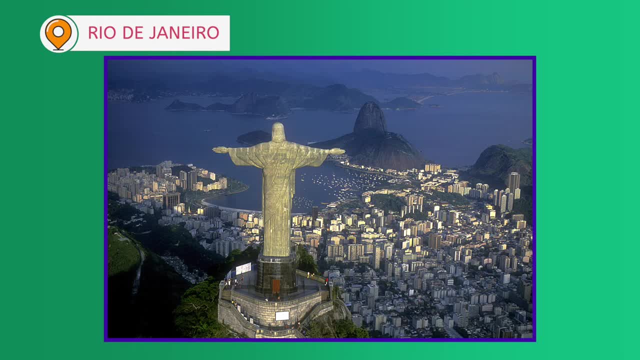 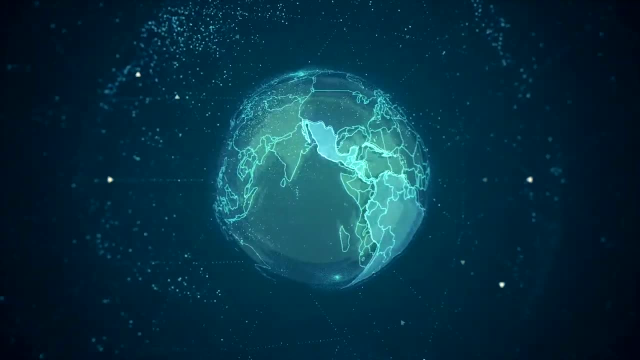 Many of South America's largest and most well-known cities are on the coast, from Buenos Aires, Argentina, to Cartagena, Colombia, to Valparaiso, Chile. One of the most interesting and most interesting cities in the world is the city of Sao Paulo. Brazil, the capital of Brazil and its third largest city by population. While many of the cities in Latin America are centuries or even millennia old, Brasilia was founded in 1960. That's right, the capital is less than 100 years old. Additionally, looking at this map, 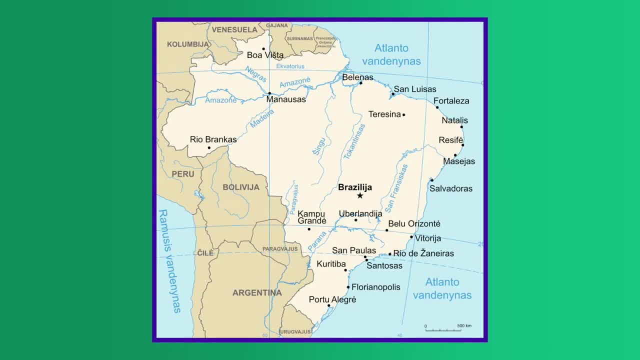 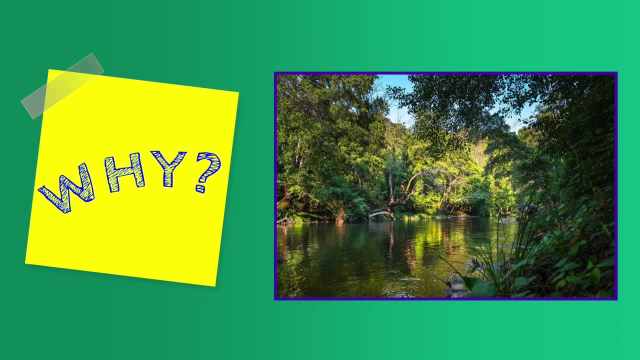 its location is far inland from the coast, an area which had been the economic powerhouse of the country. Why create a new capital out in the rainforest? Well, it was part of an experiment to bring economic power to the country, and it was part of an experiment to bring economic power to the 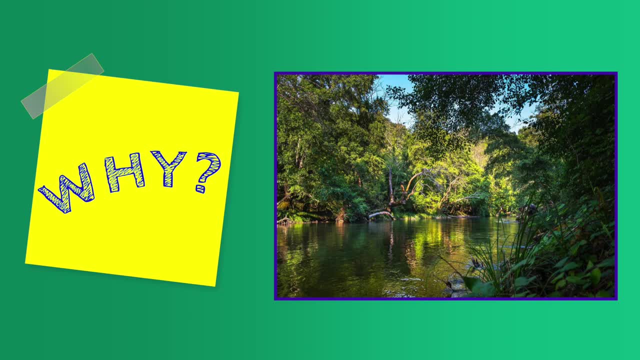 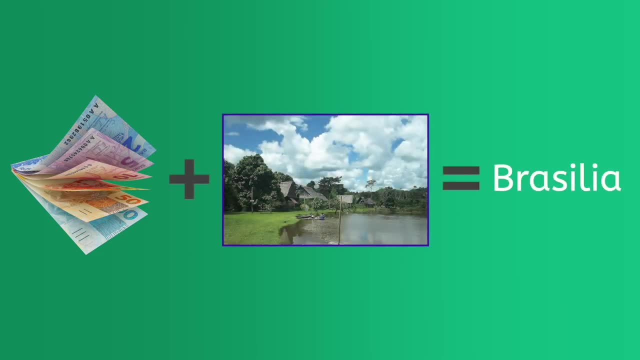 rural parts of the country by creating a forward capital or a capital city specifically moved and built to encourage economic opportunity in a less developed part of the country. As Brasilia's GDP or gross domestic product is the highest of any city in Brazil, the experiment looks pretty.